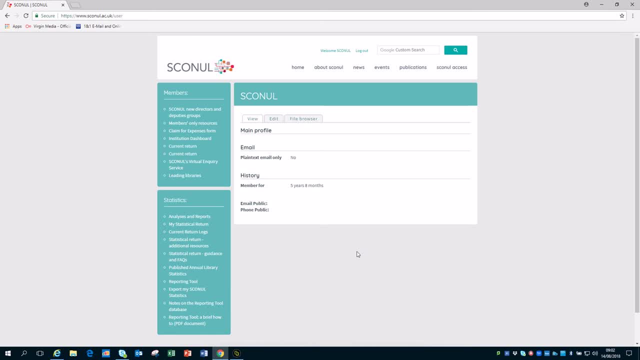 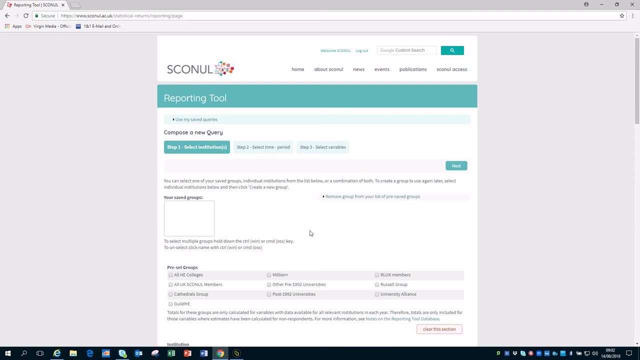 over that time. So the first thing we need to do is go to the reporting tool itself, which you can find when you log in from the welcome screen. If you look at the menu on the left hand side, you can click on reporting tool. Once you reach the reporting tool, you are guided through the three main steps of creating. 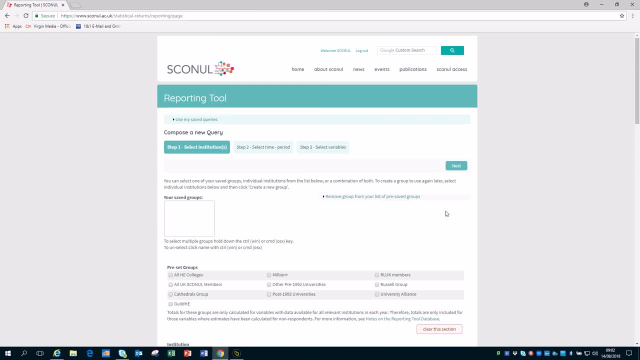 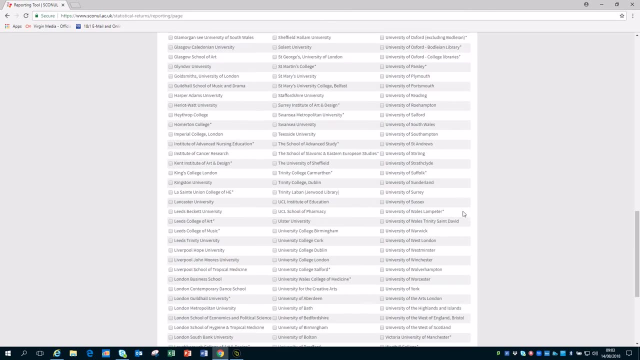 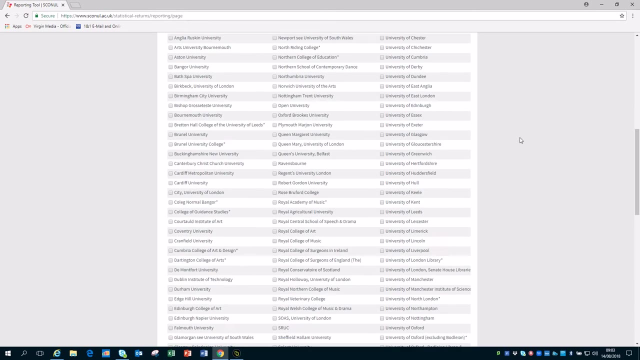 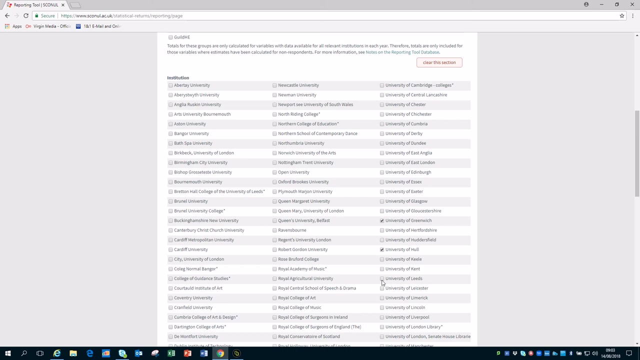 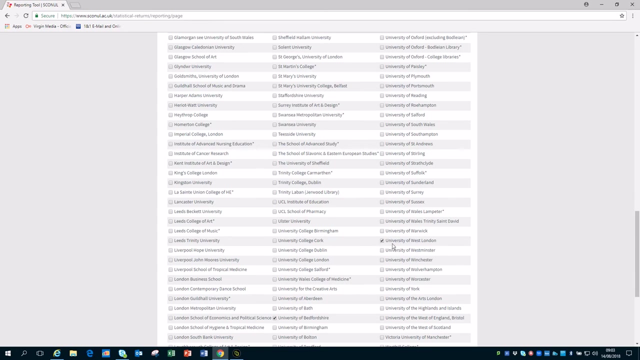 a report. To begin with, we need to select the institutions that we are interested in for this particular inquiry. So I am going to scroll down and select the University of Bedfordshire, the University of Greenwich, the University of Hull, the University of Leeds and finally the University of West London, If I then scroll to the bottom of the page. 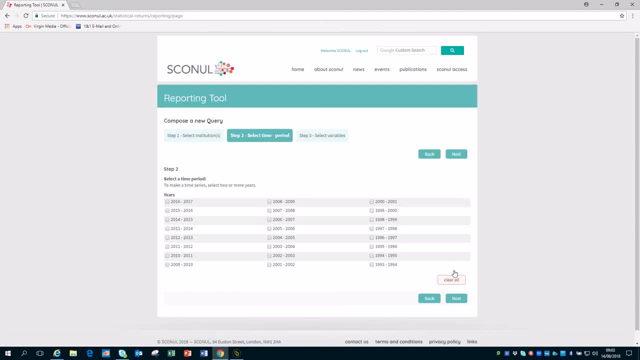 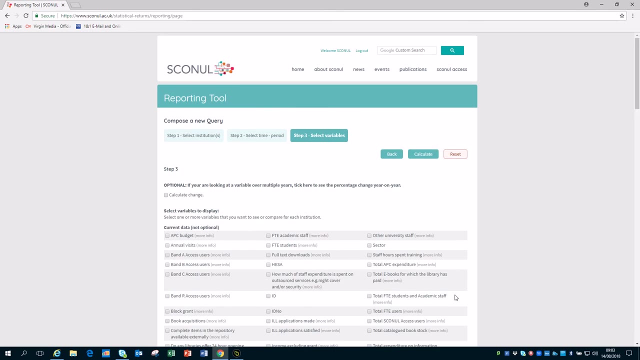 I click on next to move on to the next step. So at this point I need to select the period of time that I'm interested in. so I want to look across usage over the last three years. I then click on next again, And now I can select the actual variables I'm interested. 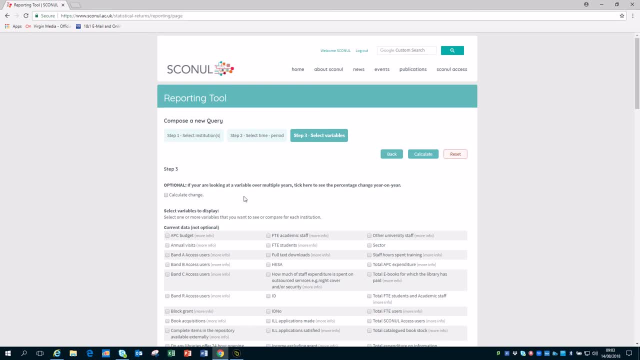 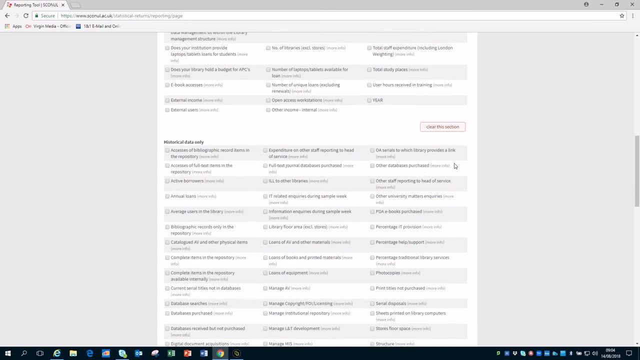 in, but I mentioned I want to look at the percentage change. so I also want to tick this box at the top so that the tool will calculate the change for me. So I'm interested in annual visits and then I want to look at how many visits per FTE student. so if I scroll to the 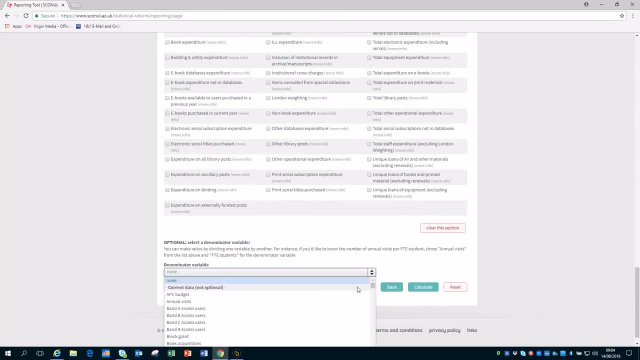 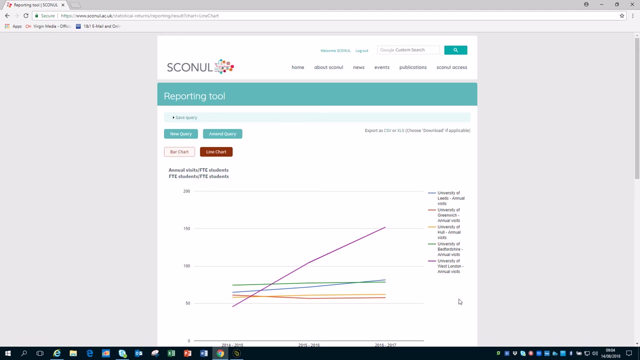 bottom I can see how many visits per FTE student. So if I scroll to the bottom, I can then select the denominator variable and scroll down to select FTE students, and I can then ask the tool to calculate this for me. So the query is run and, as you can see, I have a line chart showing me the patterns in usage. 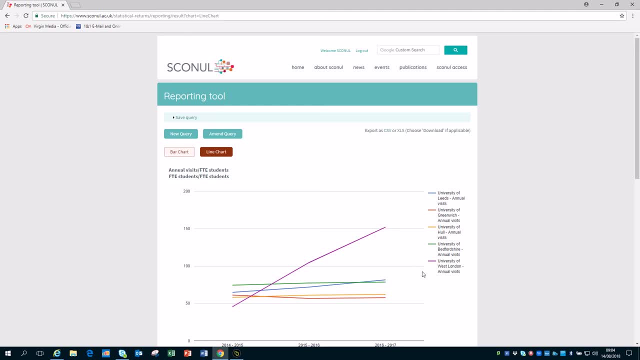 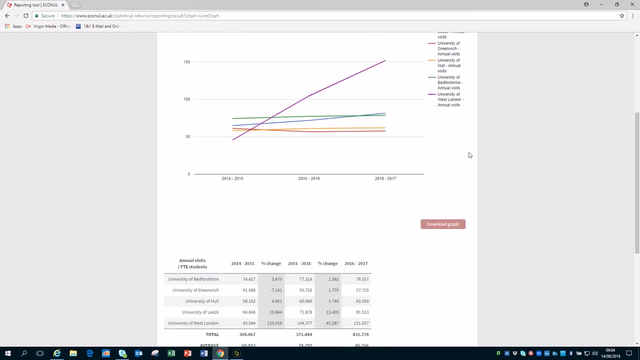 over that time for each of the five institutions that we have selected. I can also display this as a bar chart, or I could export the data in either CSV or Excel format. If I scroll down further, I can also see the actual numbers involved and in the grey column: 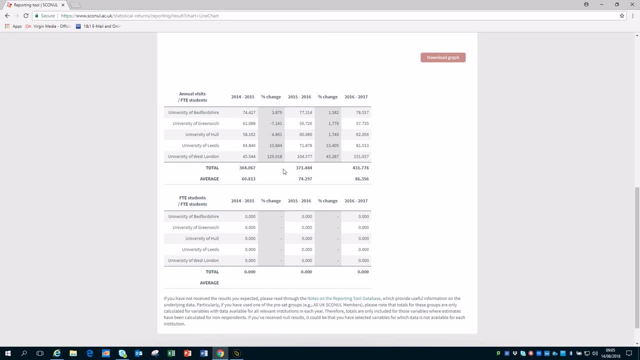 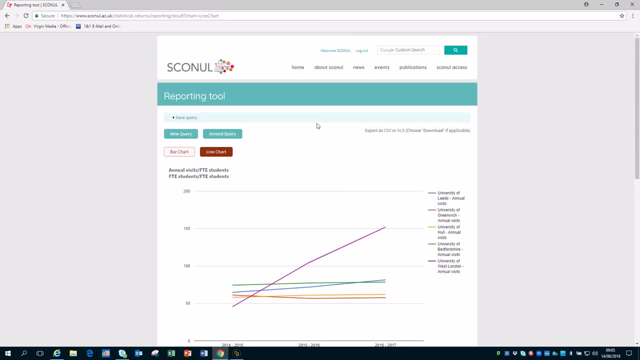 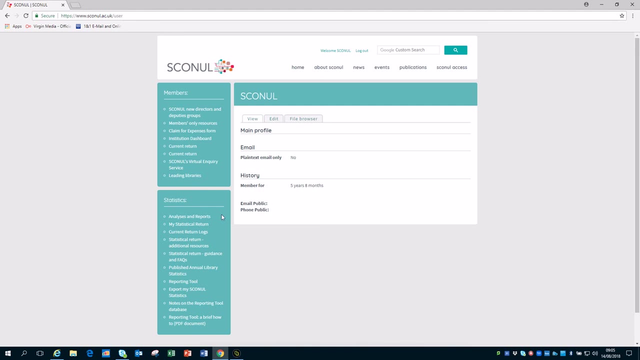 I can see the percentage change year on year. If you would like further advice about using the Scholar Statistics Reporting Tool, if we just return to the Welcome page, you can see that there is at the bottom of the left hand menu a brief guide on how to use the Reporting Tool. Thank you. 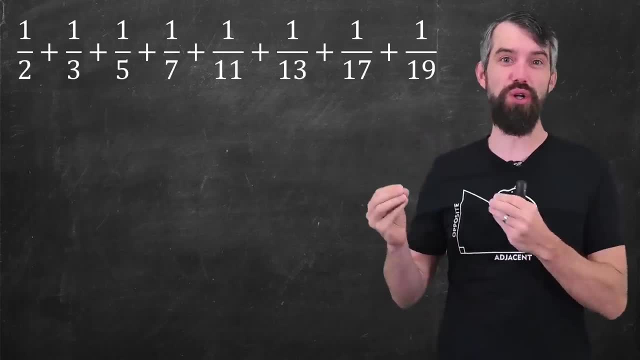 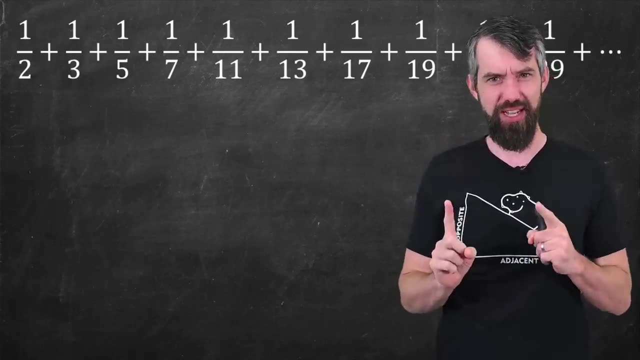 This series is the sum of reciprocal primes and the denominators are all the primes 2,, 3,, 5,, 7,, 11, and so forth. And the question is: does this series converge to a number or does it diverge to infinity? 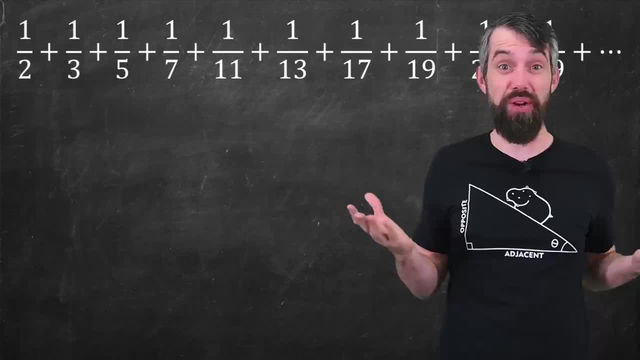 In this video, I'm going to share a delightful proof that this series of reciprocal primes actually diverges, And I'm going to be able to do this just using some standard tricks from first-year calculus. In particular, I want to contrast this series with two other, more familiar ones. 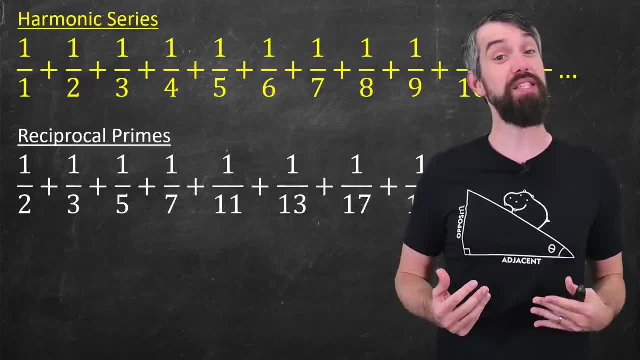 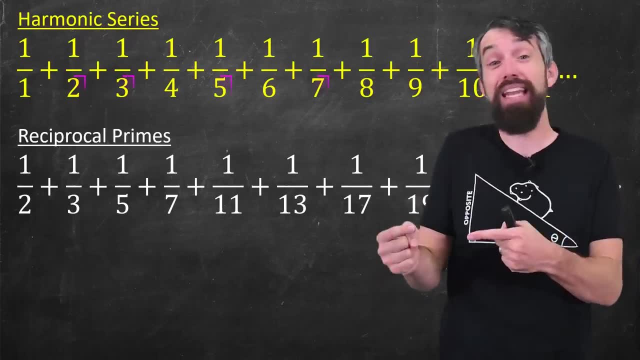 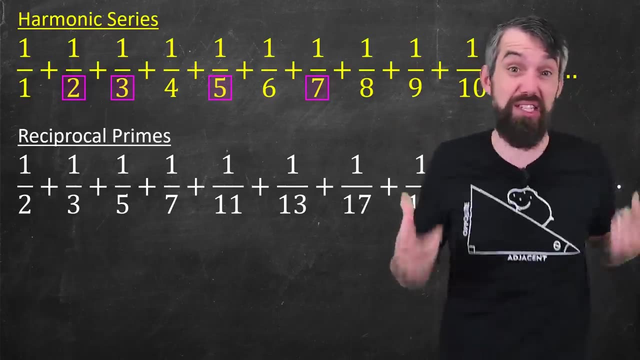 The first of which is the harmonic series. This is the sum of 1 over all of the integers. That is, the harmonic series has the primes in it, but it's got a whole bunch of other things. So the reciprocal prime is certainly smaller than the divergent harmonic series. but that doesn't tell us anything about reciprocal primes yet. 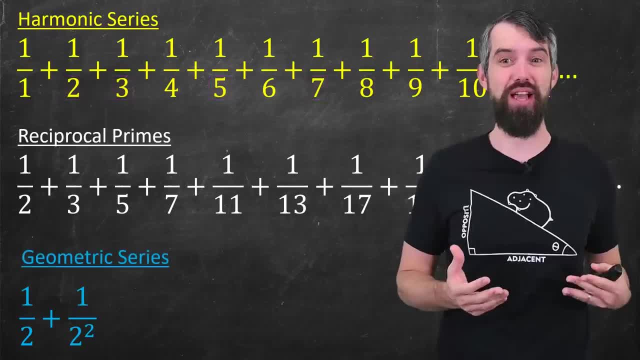 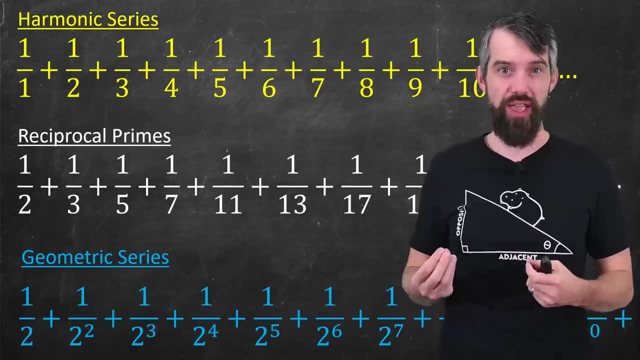 In contrast, the other really famous series from first-year calculus is the geometric series and it has expressions like one-half, one-quarter, one-eighth, one-sixteenth and so forth, And I can compare these two series as well, like they both have a half in it and then one-third is a bigger number than one-quarter.